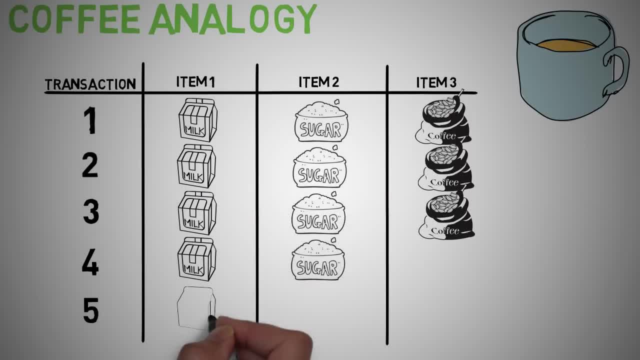 Rule 1: If milk is purchased, then sugar is also purchased. Rule 2: If sugar is purchased, then milk is also purchased. Rule 3: If milk and sugar are purchased, then coffee powder is also purchased. in 60% of the transactions. 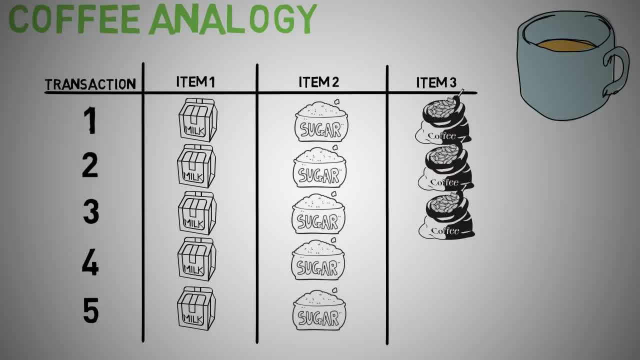 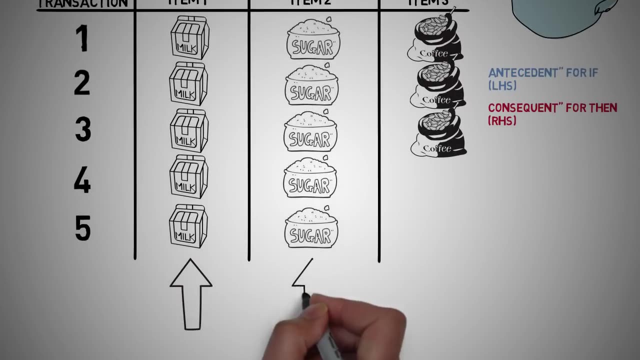 Generally, association rules are written in an if-then format. We can also use the term antecedent for if and consequent for then. From the above rules we understand the following explicitly: Whenever milk is purchased, sugar is also purchased, or vice versa. 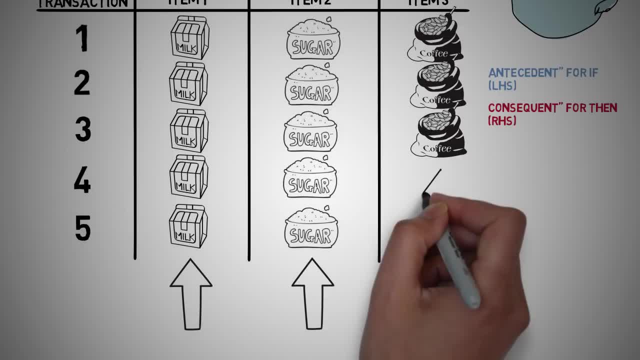 If milk and sugar are purchased, then the coffee powder is also purchased. Rule 4. If we see milk as a set with one item and coffee as a set with one item, we will use this to find sets with two items in the dataset, such as milk and coffee. 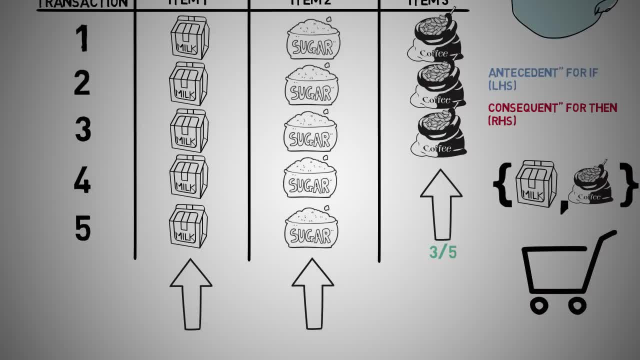 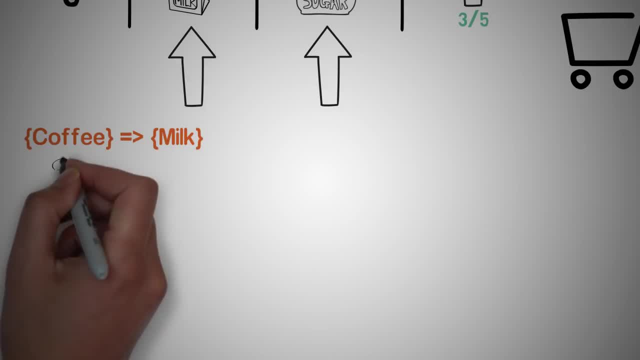 And then later we will see which products are purchased with both of these in our basket. Therefore, now we will search for a suitable right-hand side or consequent. So if someone buys coffee with milk, we will represent it as coffee to milk where coffee 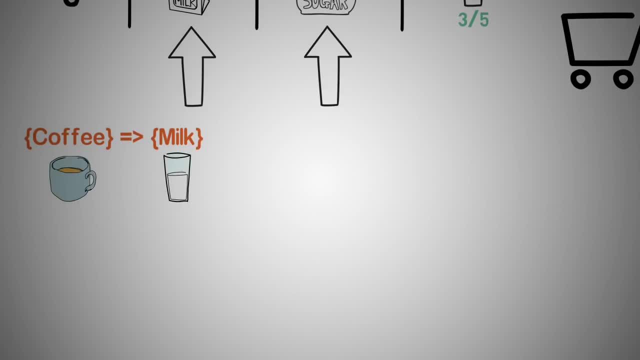 becomes the left-hand side and milk the right-hand side. When we use these to explore more K-item sets, We might find that coffee and milk to tea, Which means that people who buy coffee and milk have a possibility of buying tea as well. 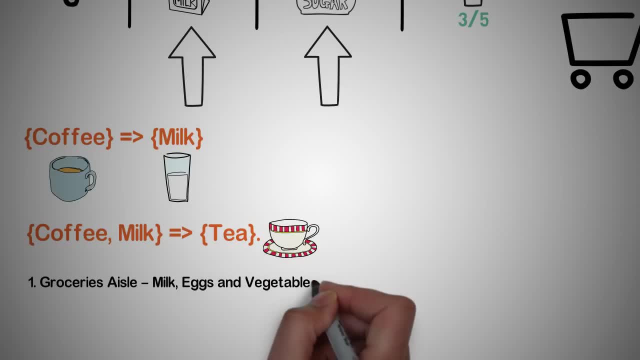 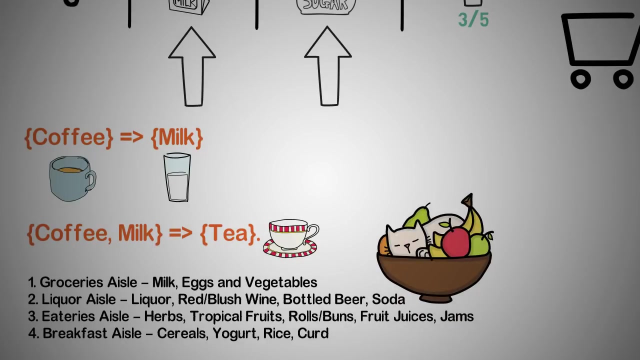 An item set is a mathematical set of products in grocery aisle: milk, eggs, vegetables, liquor aisle liquor red blush, wine, bottled beer, soda, eatery aisle herbs, tropical fruits, roll buns, fruit juices, jams and breakfast aisle cereal, yogurt, rice, curd. 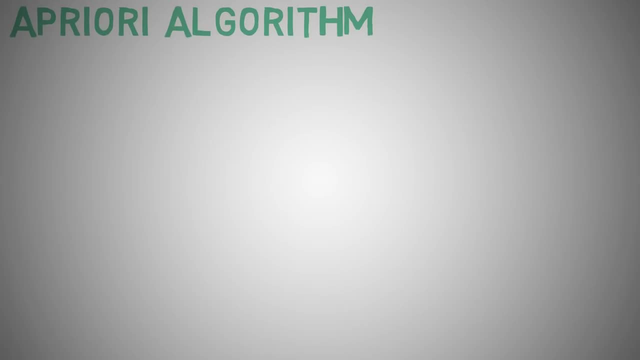 The a-priory algorithm is a clear example. The a-priory algorithm is a clear example. The a-priory algorithm is a clear example. a classical algorithm in data mining that we can use for these sorts of applications. ie recommend. 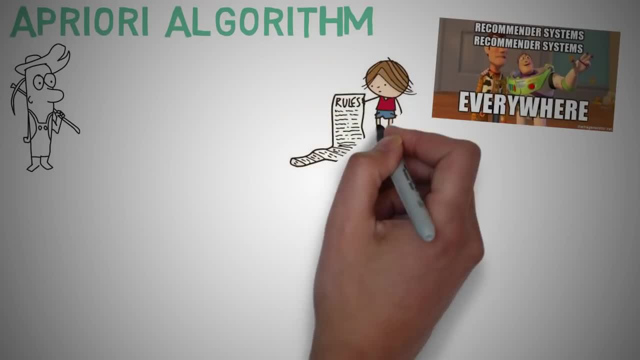 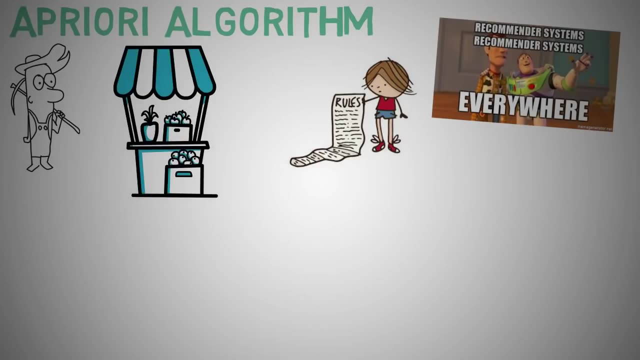 engines, so it is used for mining frequent item sets and relevant association rules. it is devised to operate on a database containing a lot of transactions, for instance items bought by customers in a store. it is very important for effective market basket analysis and it helps the customers in purchasing their items with more ease, which increases the sales of the market. 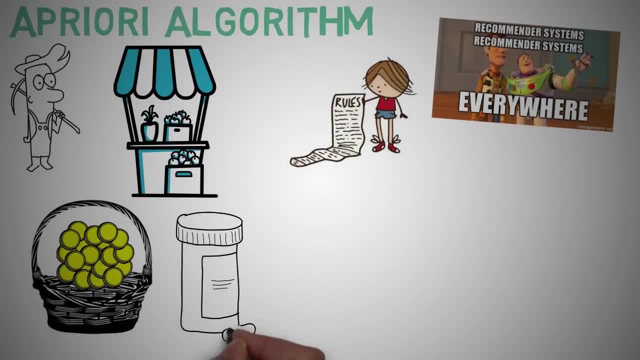 it has also been used in the field of healthcare for detection of adverse drug reactions. a key concept in a priority is to assume that all subsets of a frequent item sets must be frequent, and similarly for any infrequent item sets, all its supersets must be infrequent too. 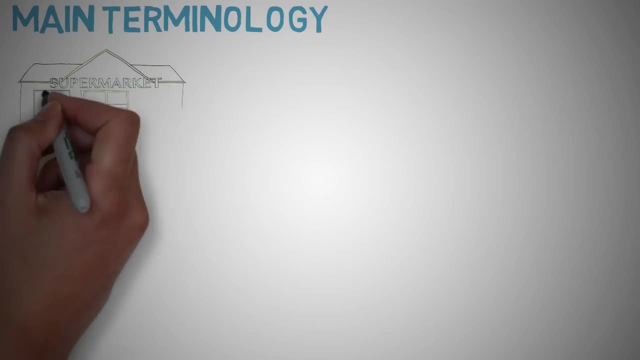 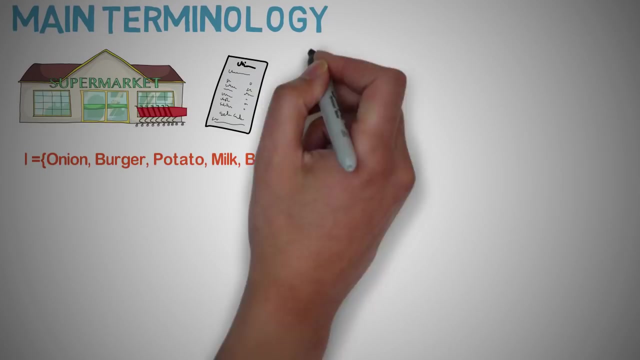 let's take another easy example from the supermarket sphere. the example that we are considering is quite small and, in practical situations, data sets contains millions and billions of transactions. the set of item set i, which contains onions, burgers, potatoes, milk and beer, and a data set consisting of six transactions. each transaction is a tuple of zeros and ones where zero represents the absence. 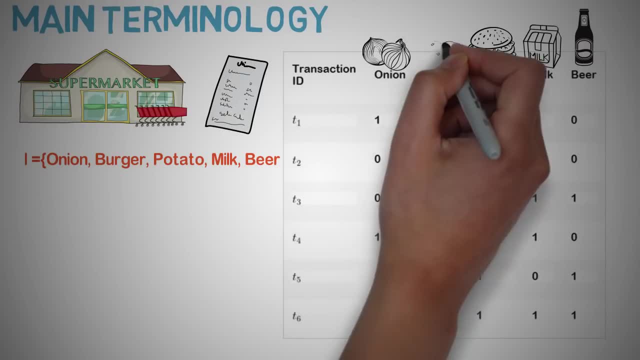 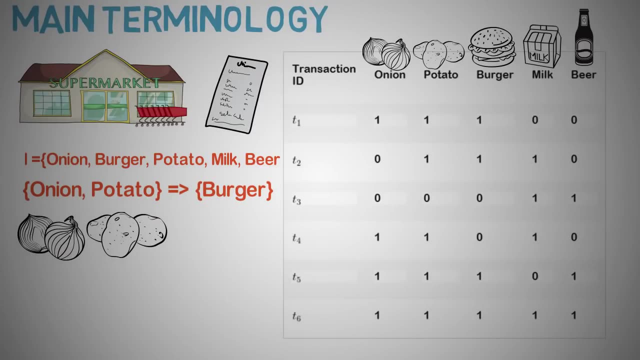 of an item and one: the presence. so far, so good. an example for the rule in the scenario would be onion and potato to burger, which means that if onion and potatoes are bought, customers also buy a burger, with no reason to collect a Bourbon bag. supposedly, there are multiple rules possible from even a small data set, so in order to select the 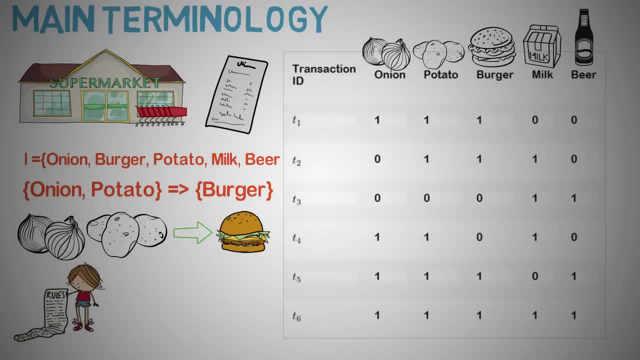 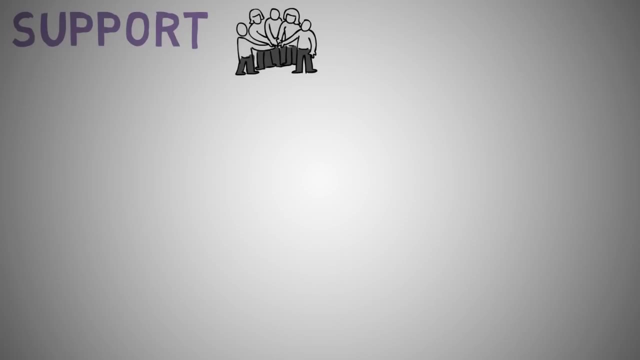 interesting ones. we use constraints on various measures of interest and significance. we will look at some of these useful measures, such as support, conference lift and conviction. the support of an item set. x is the proportion of transaction in the database in which the item x appears. it signifies the popularity of an item set. 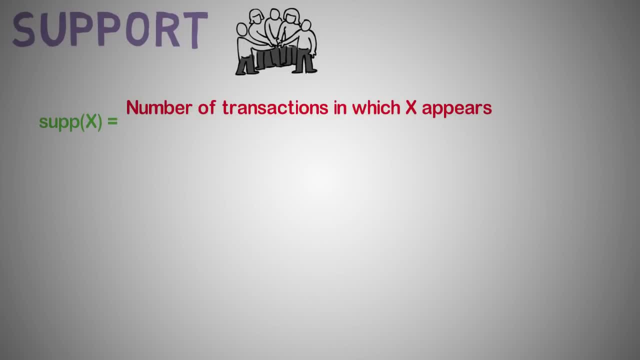 X equals the number of transactions in which X appears over the total number of transactions. In our example, the support of onions equals 4 over 6, which equals 0.6667.. If the sales of a particular item or product is a certain proportion having a meaningful 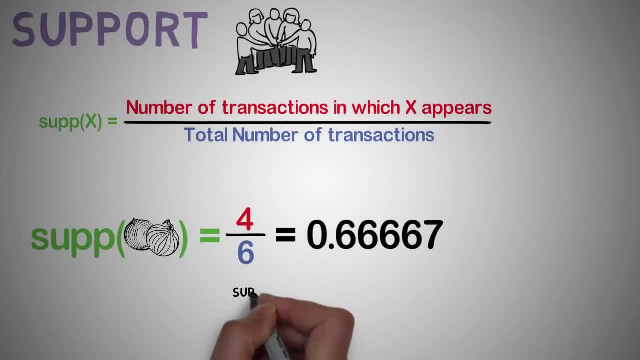 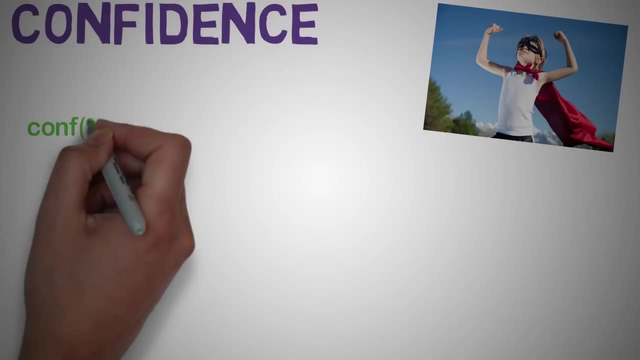 effect on profits, that proportion can be considered as a support threshold. Furthermore, we can identify item sets that have support values beyond this threshold as significant item sets. Confidence: Confidence of a rule is defined as follows: Confidence of X to Y equals the support of X union Y over support of X. 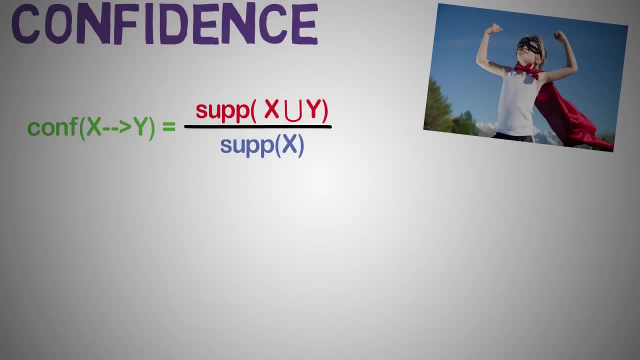 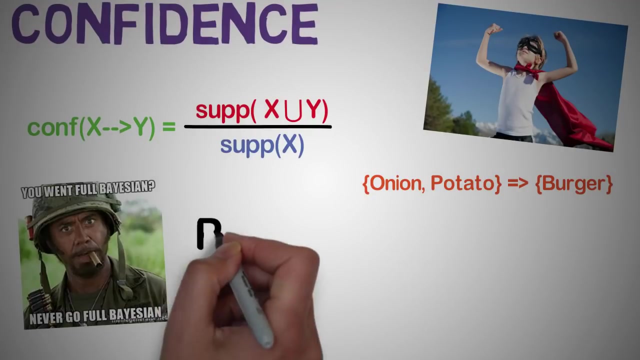 It signifies the likelihood of item Y being purchased when item X is purchased. So for the rule, onions with potatoes, and what's the likelihood of burgers being bought. So I'm sure by now you're sensing some Bayesian theory along these lines. You would be correct if you interpreted this as conditional probability, ie the probability. 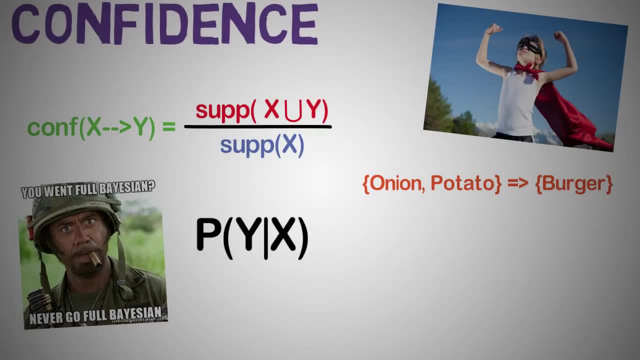 of finding the item set Y in the transactions, given the transactions already contain X. It can give some important insights, but it also has a major drawback: It only takes into account the popularity of the item set X and not the popularity of Y. If Y is equally popular as X, then there is a higher probability that the transactions 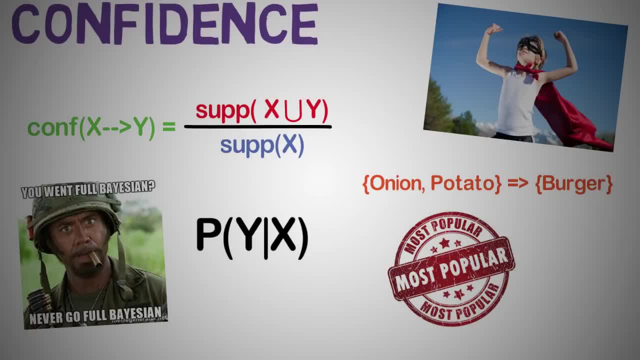 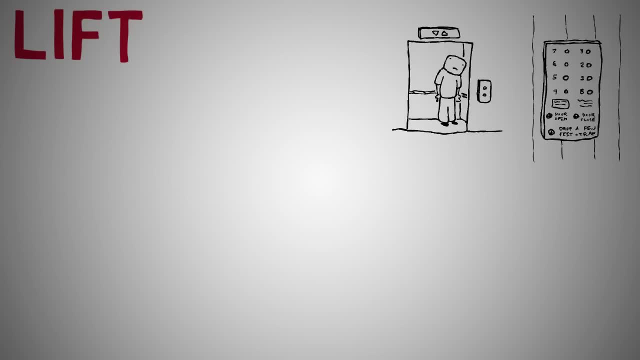 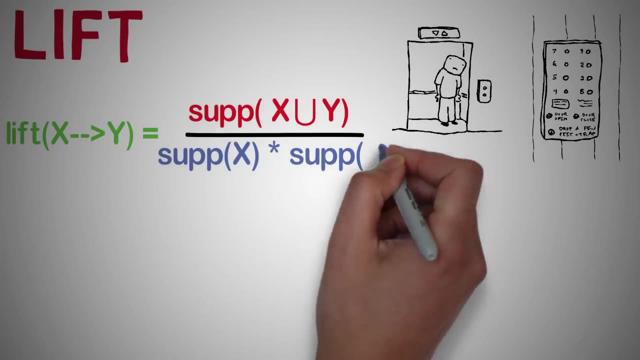 containing X will also contain Y, thus increasing confidence. To overcome this drawback, there is another measure called lift. The lift of a rule is defined as: the lift of X to Y equals the support of X union Y over the support of X, multiplied by the support of Y. 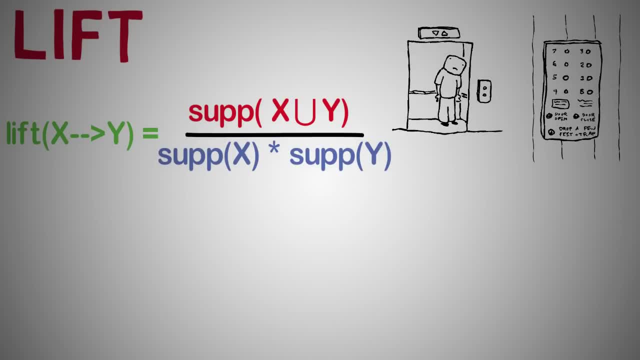 This signifies the likelihood of an item Y being purchased when item X is purchased, while taking into account the popularity of Y. In our example, if the value of lift is greater than one, It means that the item set Y is likely to be bought with item set X, while the value 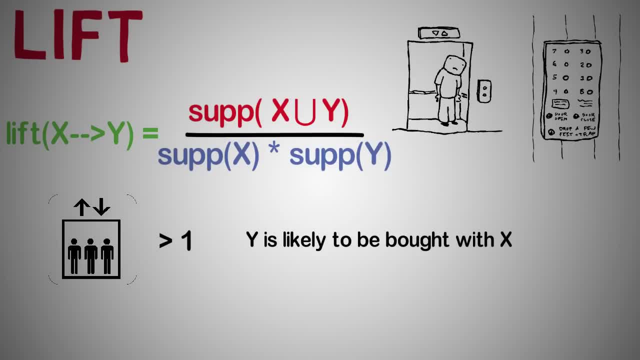 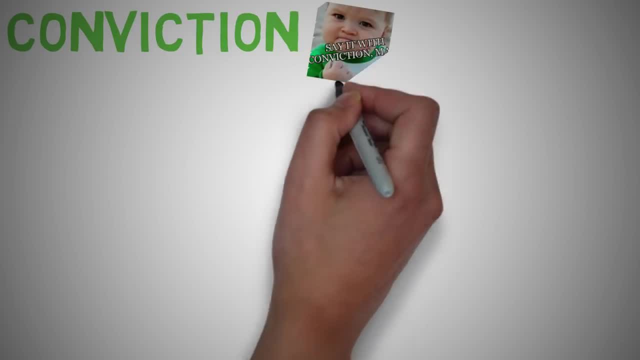 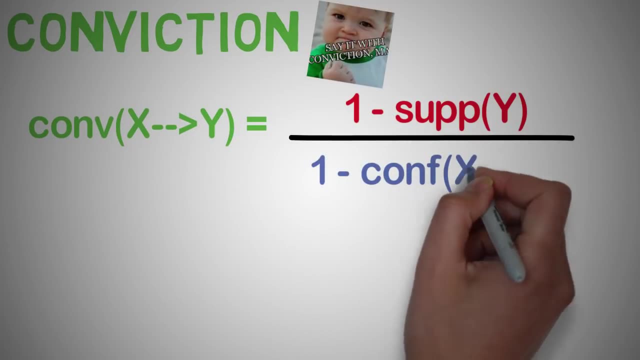 with less than 1 implies that an item set Y is unlikely to be bought if the item set X is bought. Conviction Conviction can be defined as: Conviction equals One minus the support of Y Divided by one minus Confidence of X to Y. 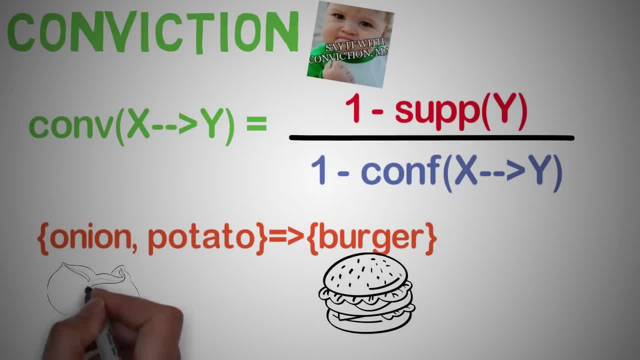 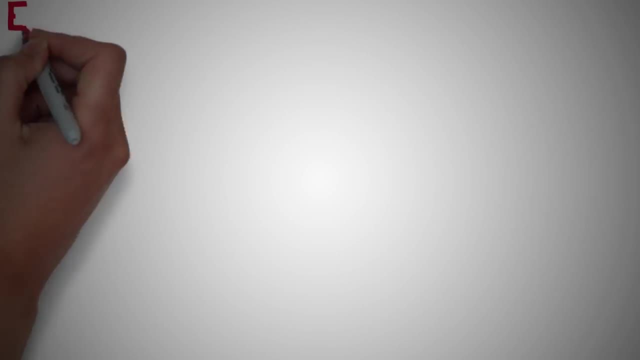 For this rule, A berger is bought, given that For language, potatoes. So the convection value of 1.32 means that the rule onions and potatoes to burgers would be incorrect 32% more if the association between x and y was an accidental chance. 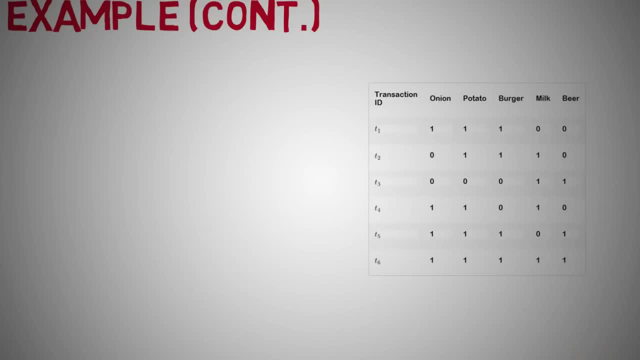 Let us now look at an intuitive explanation of the algorithm with the help of an example we used earlier Before beginning the process. let us set the support threshold to 50%, meaning that those items are significant for which the support is more than 50%. 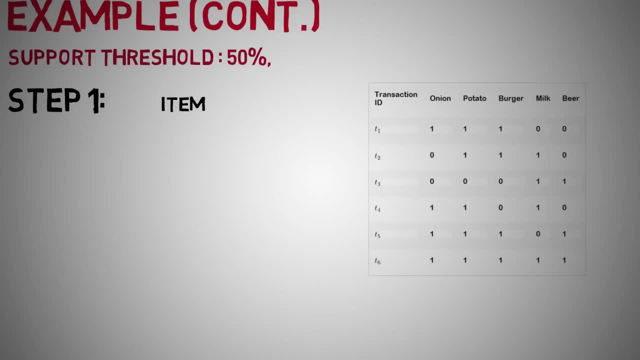 So step 1, we create a frequency table of all the items that occur in all the transactions, based on our dataset. So for our case, we can see that onions we have a frequency of 4, potatoes 5, burgers 4, milk 4 and beer 2.. 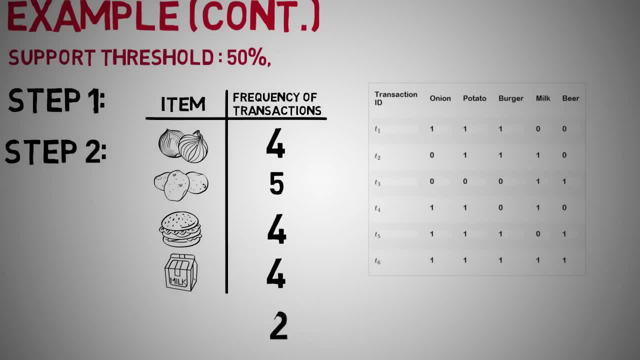 Step 2, we know that only those elements are significant for which the support is greater than or equal to the support threshold. Here the support threshold is 50%, Hence only these items are significant which occur in more than 3 transactions, and such 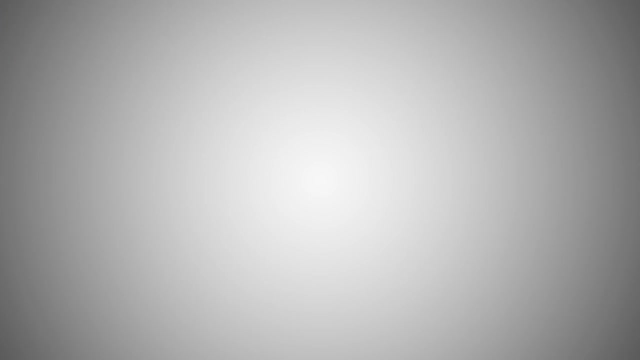 items are onions, potatoes, burgers and milk. Step 3, the next step is to make all the possible pairs of the significant items, keeping in mind that order doesn't matter, which means that AB is the same as BA. To do this, take the first item and pair it with all the others, such as onions and potatoes. 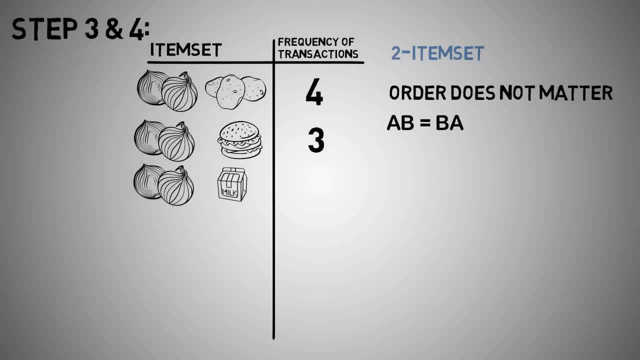 onions and burgers. Similarly considering the second item and pair it with the preceding items, which means potatoes and burgers and potatoes and milk. We are only considering the preceding items because potatoes and onions, which is the same as onions and potatoes, already exist. 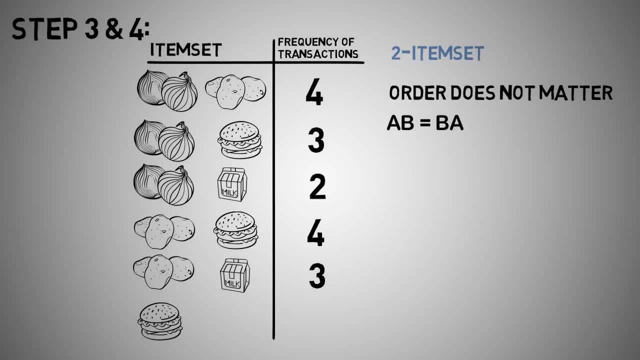 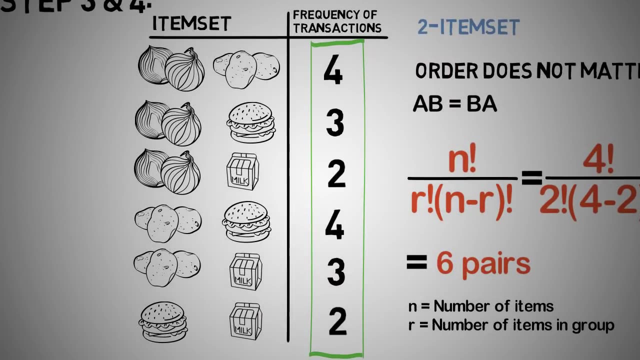 So all the pairs in our example are: onions, potatoes, onions, burgers, onions, milk, potatoes and burgers, potatoes and milk and burgers and milk. We essentially calculate the combination. Step 4, we will now calculate the occurrences of each pair in all the transactions. 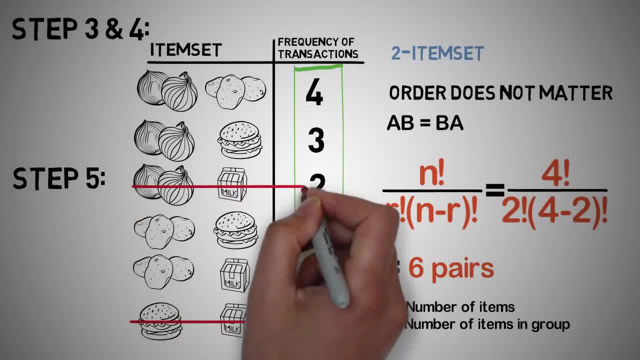 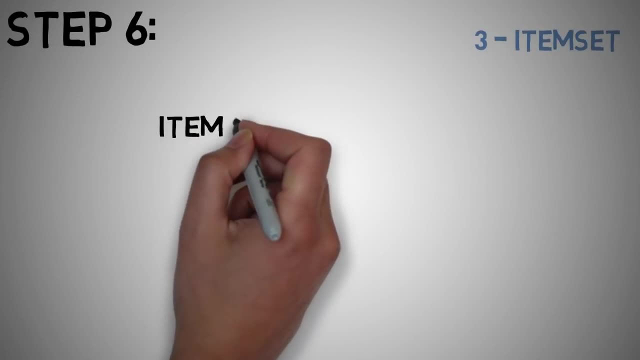 Step 5, again, only those significant item sets which cross the support threshold are passed through. These are onions and potatoes, onions and burgers, potatoes and burgers and potatoes and milk. Step 6, now, let's say we would like to look for a set with 3 items that are purchased. 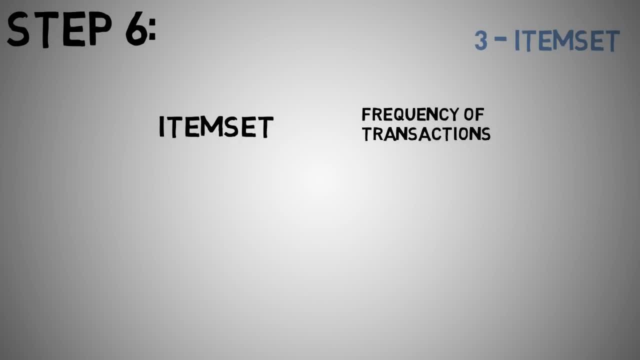 together. We will use these items as found in step 5 and create a set of 3 items. To create a set of 3 items, another rule called self join is required. It says that from the item pairs: onions, potatoes, onions, burgers, potatoes, burgers and potatoes. 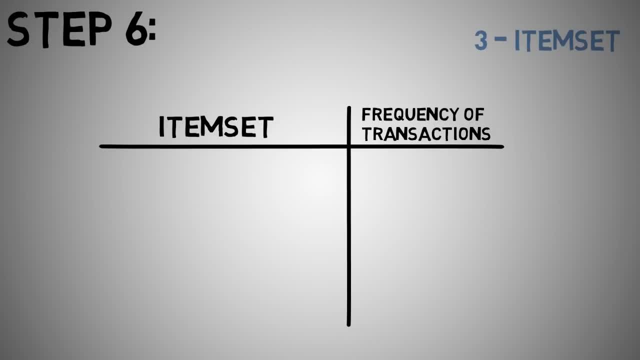 milk. we look for pairs with the identical first letter, and so we get onions, potatoes and onions burgers. this gives onions, potatoes and burgers, and then we have potatoes, burgers and potatoes and milk. Next we find the frequency for these two item sets, and then we get 3 for onions potatoes.